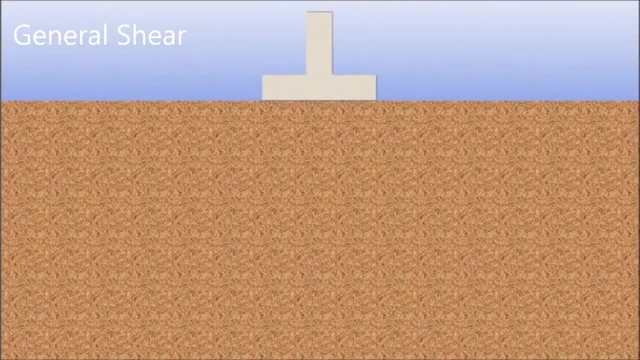 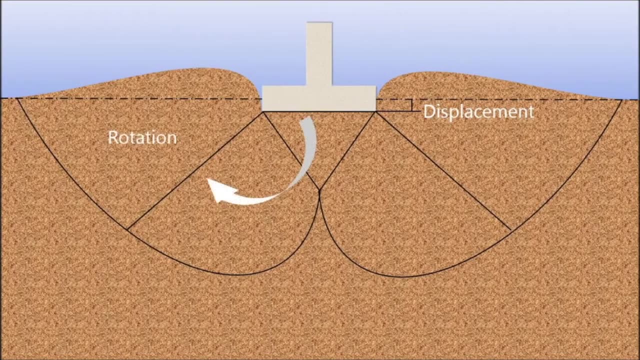 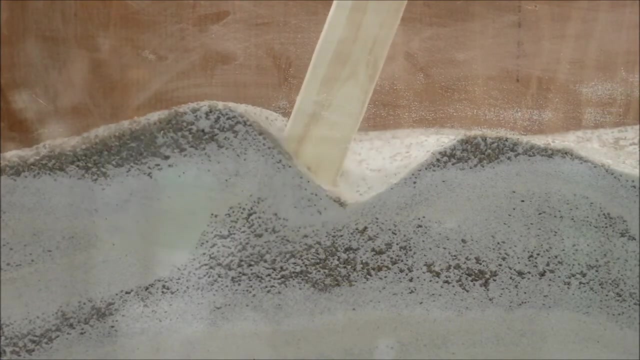 and movement along the shear plane. General shear failure occurs in dense, cohesionless soils and undrained cohesive soils. General shear failure is characterized by a well-defined shear plane with clear disturbances in the surface soils. This type of failure occurs suddenly and can cause significant rotation of the structure. 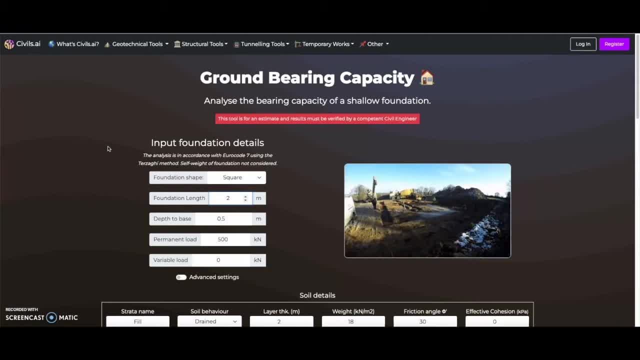 So let's look at how Civil's AI can help us to predict foundation bearing capacity. In the first section, we can control our foundation size and applied loading transferred to the foundation. We can select foundation shape, the size of the foundation, the depth to the base of. 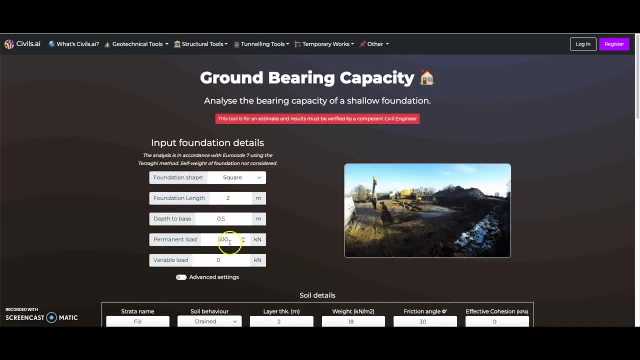 the foundation and the magnitude of the loading applied. There are also advanced features for users with more experience of the software. For example, we can control the size of the foundation and the depth to the base of the foundation. Here you can adjust the soil layer name. 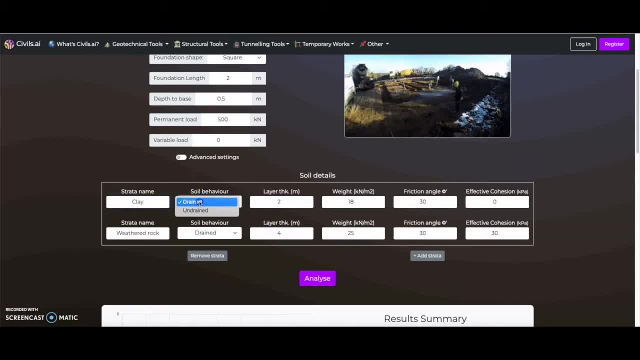 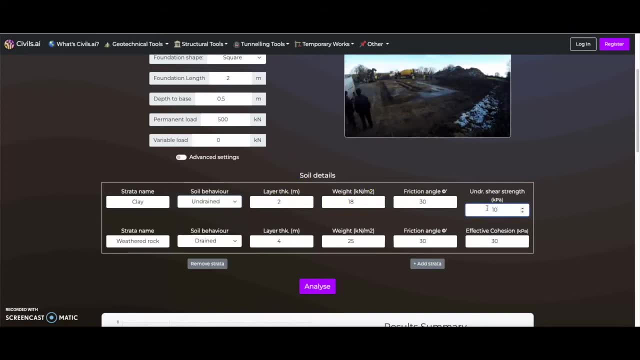 Control whether the soil behavior is drained or undrained. The thickness of the layer and soil properties can also be fine-tuned here. Soil layers can be added or removed with the buttons at the bottom. After you've input your parameters, you can hit analyze or the enter key to generate. 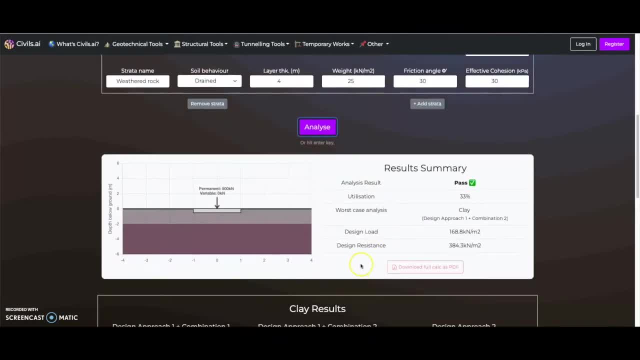 results. Our results will show whether this section passes our checks. If the section passes our checks, the design will be changed. If the section passes our checks, the design will be changed. If the section turns black, the section is empty. we can end up with a clean child or injuring Skin. 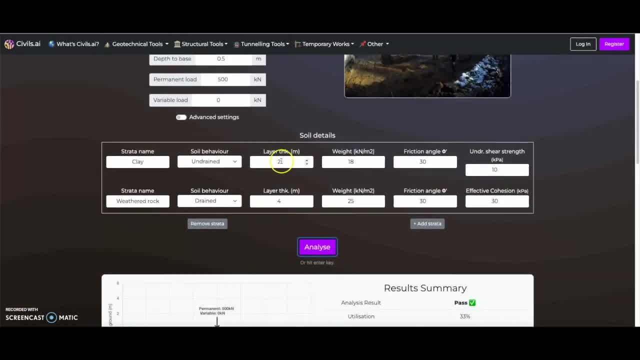 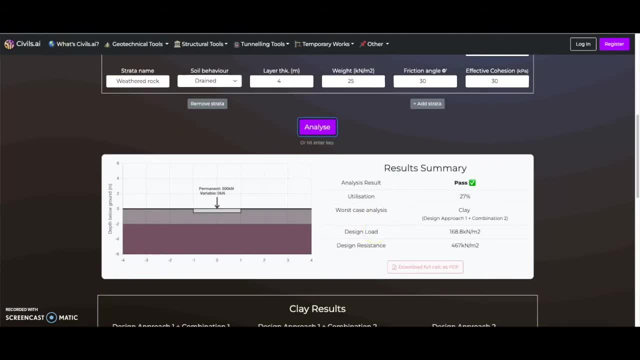 As cold air inside the material becomes harder, we can change the design and see whether the design has changed or not. In the next section we can see how a temperature change of the temperature contains the dielectric resistance, which is divided into two. The K- eldest is based on an. 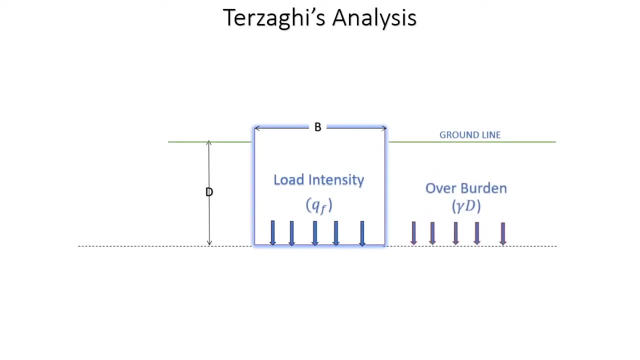 ultraviolet planet on the x-axis tweets. results are more accurate and meaningful. We can quickly adjust properties throughout the calculation to understand the nature of the model. Next up we can level and a. width, b, A, load intensity. QF is applied to the soil at the base of the foundation. 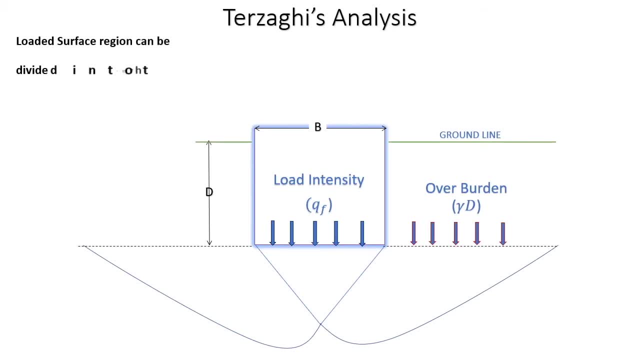 along with any additional overburden. This calculation only considers the general shear failure case, which is divided into three zones. The punching shear zone is located directly below the foundation. The radial shear zone is located from the edges of the foundation outwards. The linear shear zone is located outside the bounds of the radial shear zone.